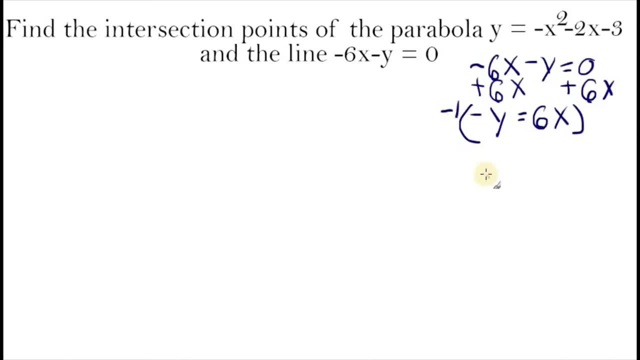 going to multiply the whole thing by negative 1. So the y will change to a positive and the 6x will change to a negative. Now we're going to plug this answer into the parabola equation. We're going to write down negative. 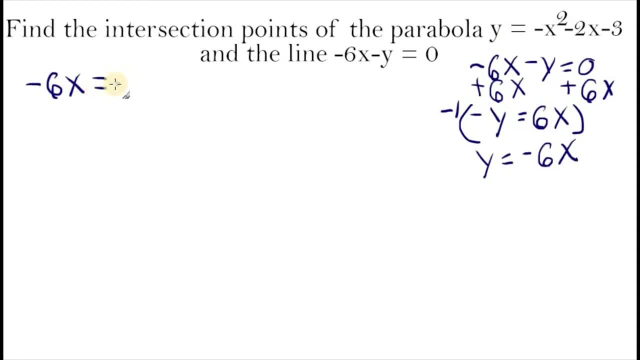 6x is equal to negative x squared minus 2x minus 3.. We're going to add 6x on both sides And you'll end up with negative x squared plus 4x minus 3.. We're going to change the. 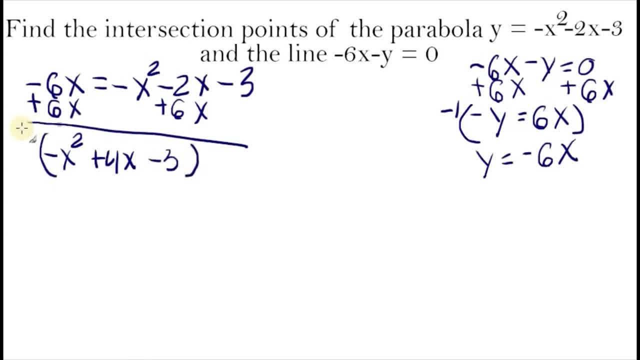 negative x squared to a positive. I'm multiplying everything but negative 1, you'll get x squared minus 4x plus 3.. And now all we have to do is factor. So I'm going to create two such parentheses, with x in each one, because x. 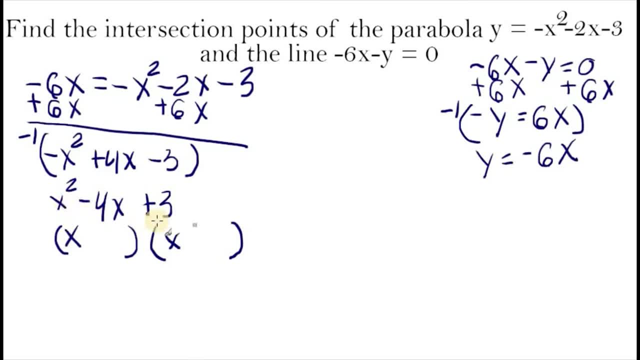 times x equals x squared. And now we need to find what number, what two numbers will multiply to be 3, but add to be negative 4.. You can do negative 3, negative 1.. If you get negative 3 times negative 1, it will equal positive 3. And negative 3 plus negative 1. 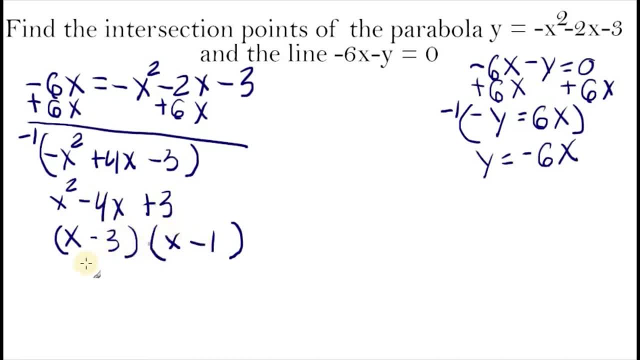 will equal negative 4. You can check it by going through and factoring, But we're just going to continue, So I need to solve for each of these two x's. So I'm going to set them both equal to 0. So x minus 3 equals 0. And x minus 1 equals 0. So over. 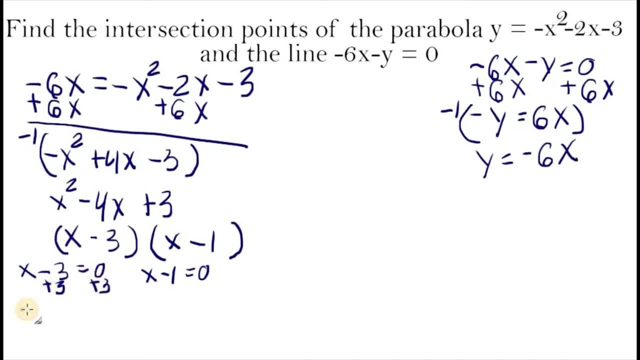 here. I'm going to add 3 on both sides, And I'll get x is equal to 3.. I'm going to add 1 on both sides. for this one. I'm going to get x is equal to 1. And I'm going to add. 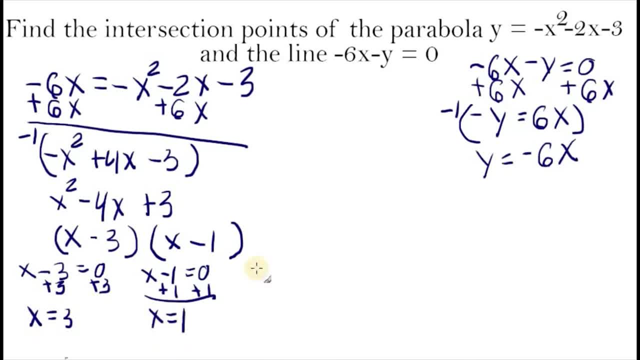 1 on both sides for this one. Now that we've solved for x, we need to find out what y is. It wants to know the points on the graph. So we're going to take this equation that we've already solved, where it says y equals negative 6x, and plug in each of these numbers.